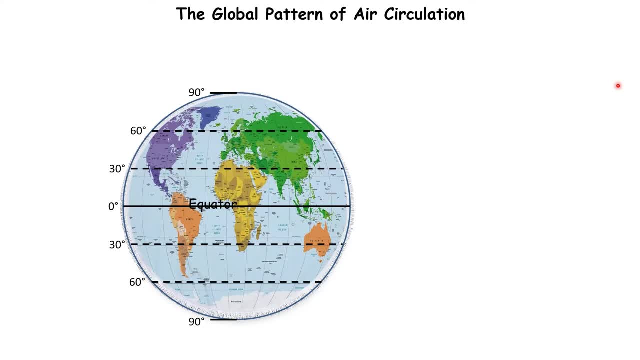 So let's move on and let's have a look at what this global pattern of air circulation is. Now, we've said, the sun's rays are concentrated where the Equator is, So it is warm there. Therefore, air rises above the equator. 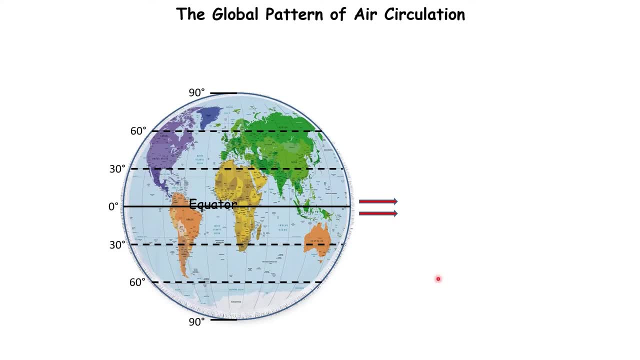 When it rises up high within the atmosphere, it will spread out. It moves out to each side because it can't go out into space. So as it gets higher it will move out from where it's rising from Now also as the air rises in the atmosphere. 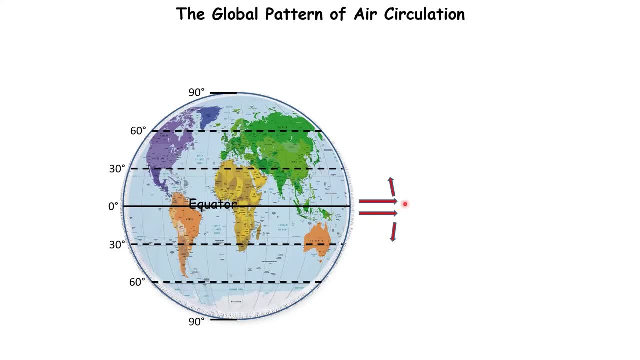 it gets colder. For every 100 metres in height you go up it gets one degree centigrade colder. And cold air doesn't rise, cold air sinks. So this air that has moved out away from the equator, it sinks back down, And the places where it sinks back down are about 30 degrees north of the. 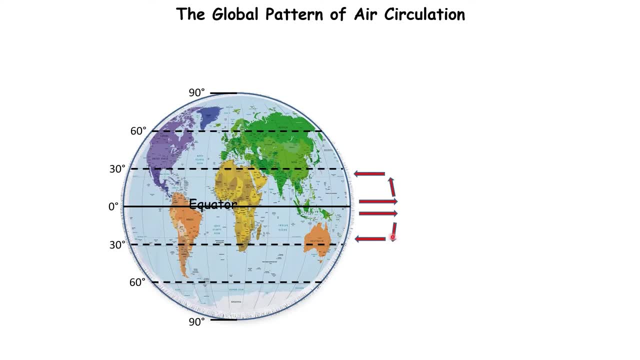 equator and 30 degrees south of the equator. As the air sinks down, it will move away from these areas, forming two cells, like so that we call the Hadley cells- Now at 90 degrees north, where the North Pole is, and at 90 degrees south, where the South Pole is. it is very cold. 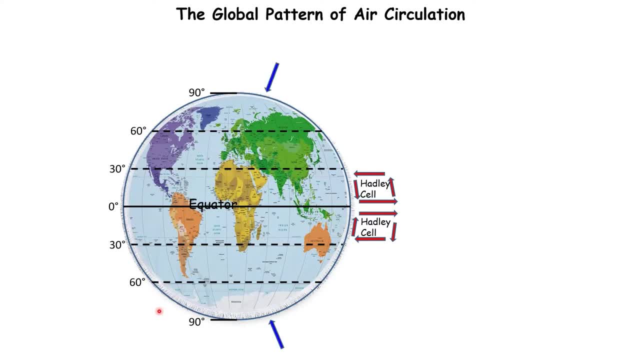 Therefore, in these areas, air sinks. The air sinks down towards the ground and when it meets the ground, it will spread out away from the ground. Yes, it will go this direction as well and this direction as well, but for the sake of 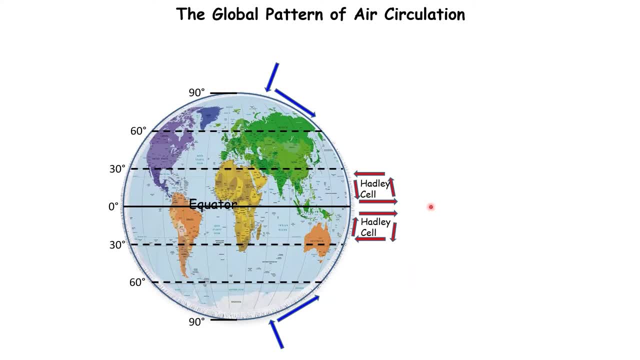 this diagram. I'm just showing you where the air is going on the right on the east side of this map that you can see, As the air moves away from 90 degrees towards the 60 degrees line, it will be getting warmer as it moves away from the North Pole. Now, as the air moves away from the north, 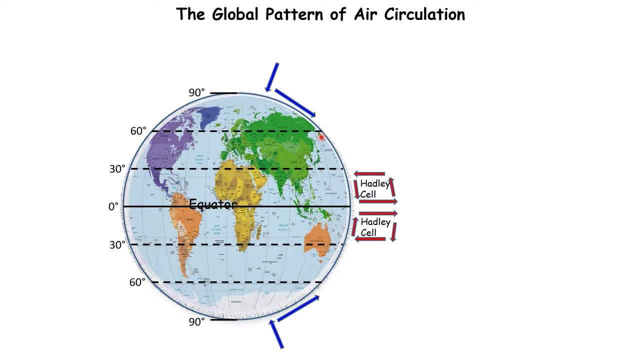 pole here, And therefore, as it gets warmer it will rise. And here, as the air moves from 90 degrees south up to 60 degrees south, here it will be getting warmer as it moves away from Antarctica and then it will become less dense and it will rise again. These cells also rotate their air. 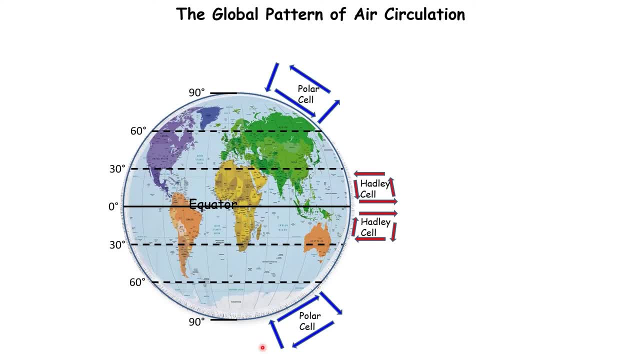 and these ones are called the polar cells. Now this updraft, this moving up of air here will drag up air next to it. So there we go, And this air beside it is being dragged up, And this downwards movement of air in the Hadley cell at 30 degrees south, and this downwards. 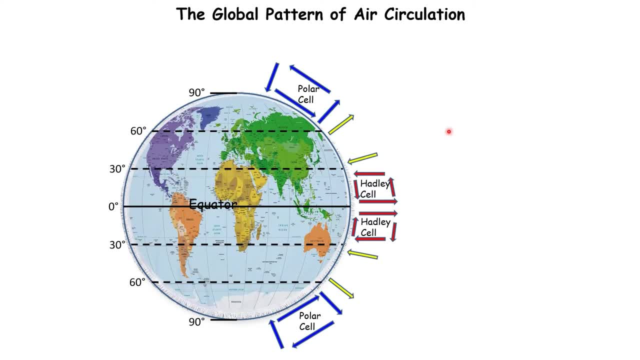 movement of air here at 30 degrees north, that will drag air down with it, And then we can complete these two cells, and these are called the ferrule cells. Now, what we can see here is the global pattern of air circulation. This is the way that air moves. 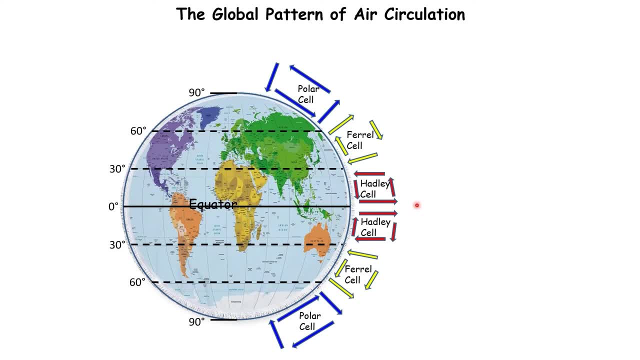 around the planet, But if we look, we've got definite areas where the air is rising. It's rising here at 0 degrees. It's rising here at 60 degrees And, as we know, rising air will lead to clouds forming and rain falling. So we can see that the air is rising here at 60 degrees. 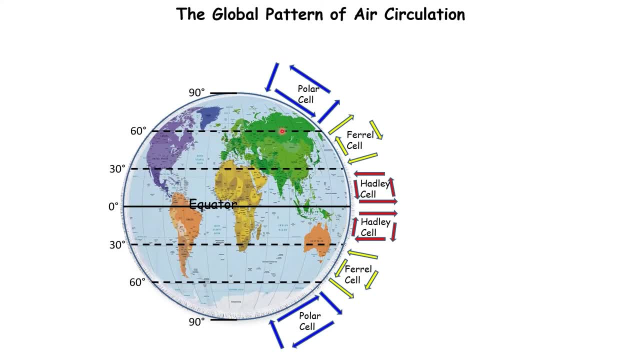 And that's what we're looking for. So this explains why Britain is quite a wet country, Because it's found at 60 degrees north, where you get this low pressure. This explains why at the equator it is so wet, Because you have low pressure, And likewise it's 60 degrees south. 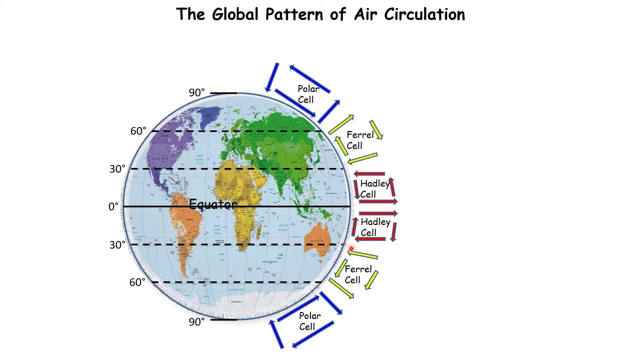 We also have areas where air is sinking. So here at 30 degrees south, here at 30 degrees north, And along these lines you get a line of deserts such as the Sahara desert, such as the Atacama desert and such as the Gobi desert in China. here 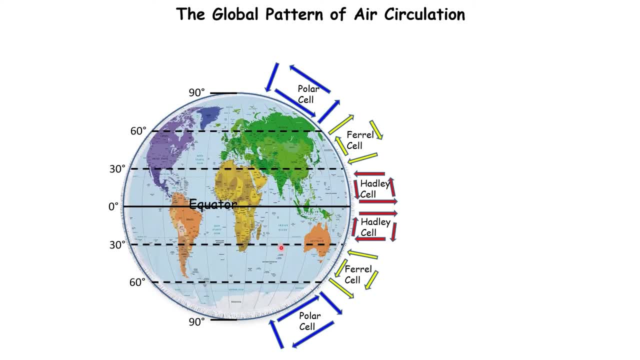 and these deserts form because this sinking air, which is high pressure, means that clouds don't form. Antarctica some people describe as the largest desert, largest desert on the planet, and it's because here, where Antarctica is, you have sinking air which is high pressure. likewise in the Arctic, you've got 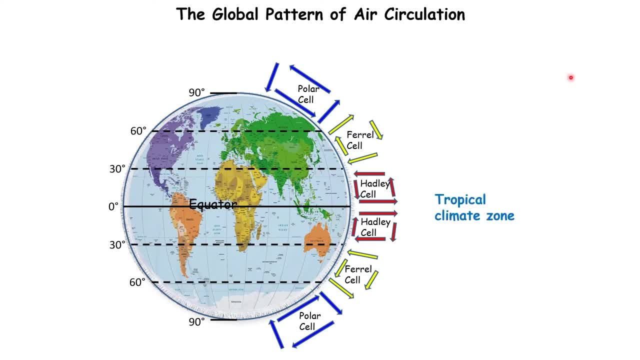 sinking air, which is high pressure. now, each of these areas where you get rising air or sinking air is known as a different climate zone. so here, at nought degrees, it's the tropical climate zone. at 30 degrees north and 30 degrees south, where the deserts are, we call them the subtropical climate zones. at 60 degrees,